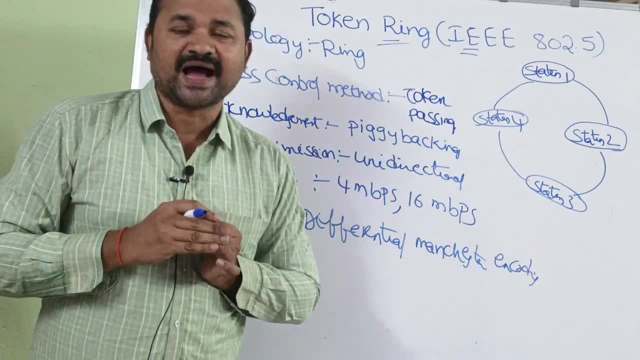 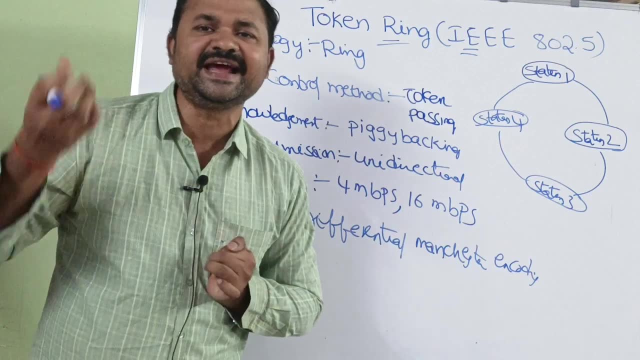 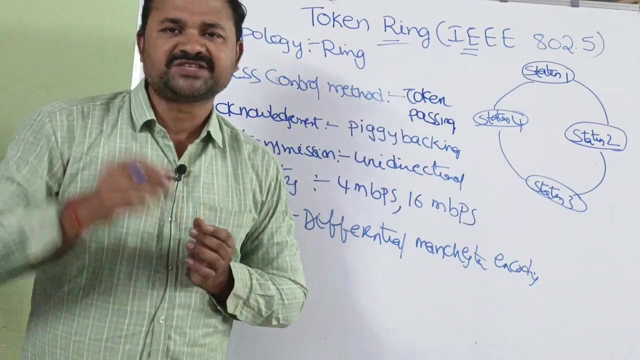 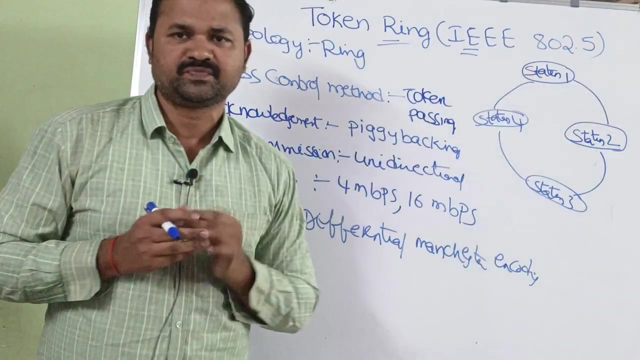 Then station one must wait until it gets the token. So after acquiring the token, only station one can send the data. So let us assume that now station one has some data as well as station one has a token. So now station one can send the data. So after sending the data, the corresponding 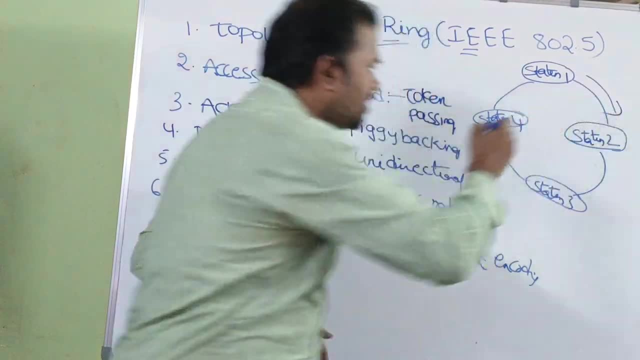 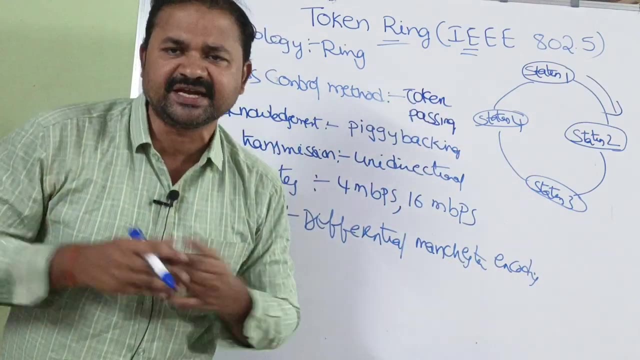 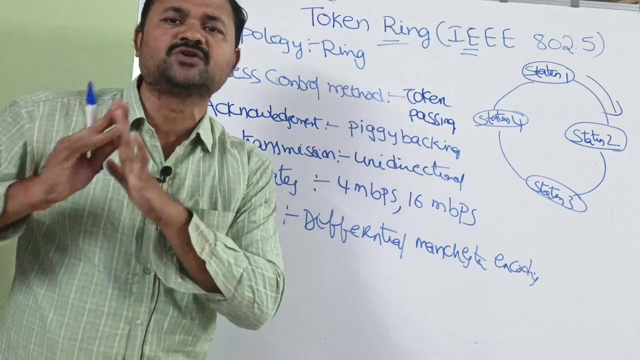 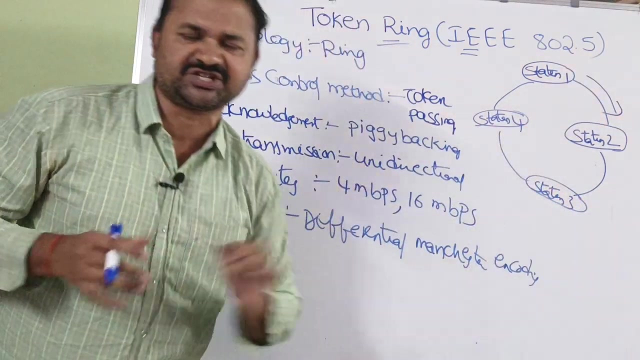 token, the corresponding token will be passed to its next station. suppose if station 2 has some data to send now, station 2 can send the data. now. suppose if station 2 has no data to send, then station 2 simply passes this token to its next station. so here we don't have any collisions. 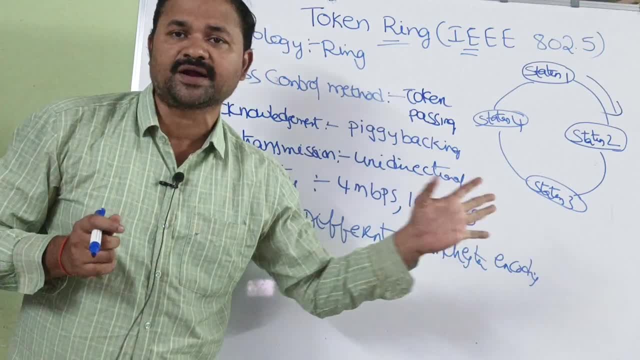 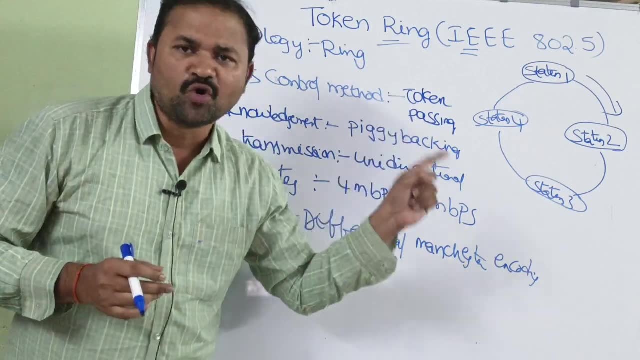 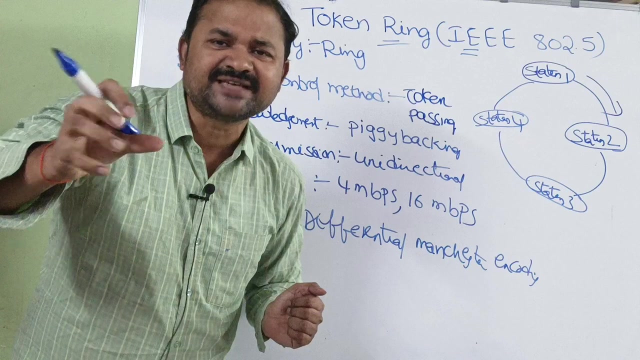 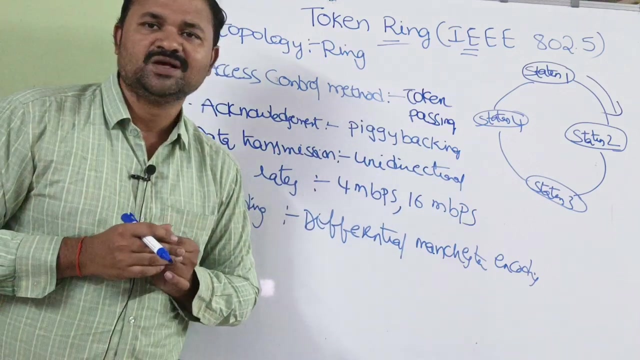 why? because here multiple stations are not trying to transmit the data simultaneously, so here at a time only one station can send the data. so that means, if station one is trying to send the data, then no other stations are allowed to transmit the data. so we don't have any collisions here. so that that is about. 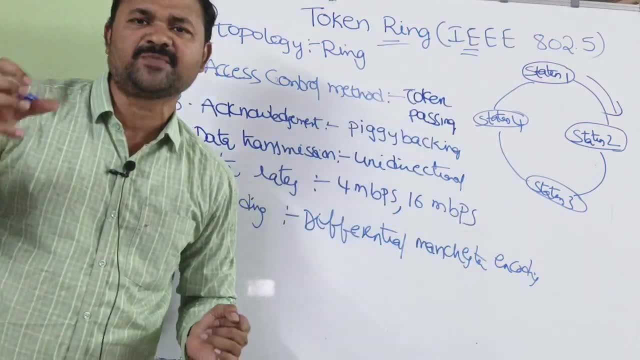 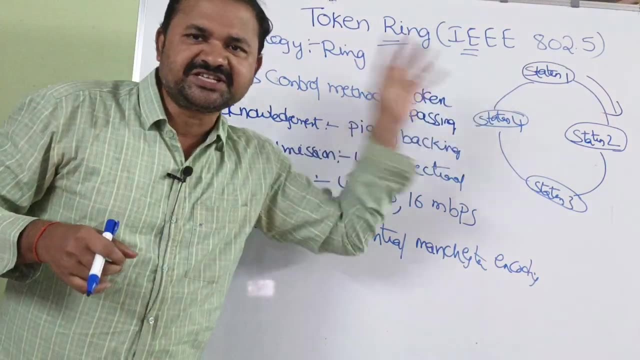 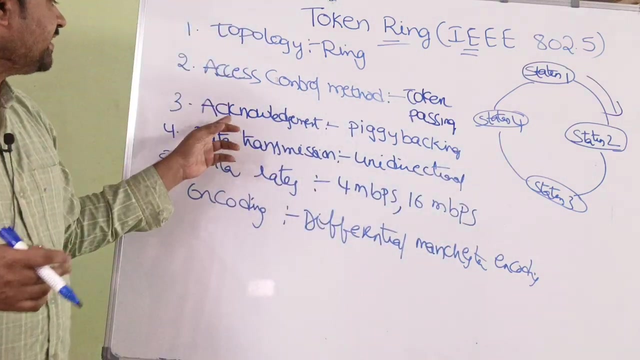 what is a token passing? so here we have a special frame called token, so that token will be circulated around the ring. okay, so if if a station has some data, then if it has the token, then it can transmit the data. okay, and uh, third one is acknowledgement. so here we follows. 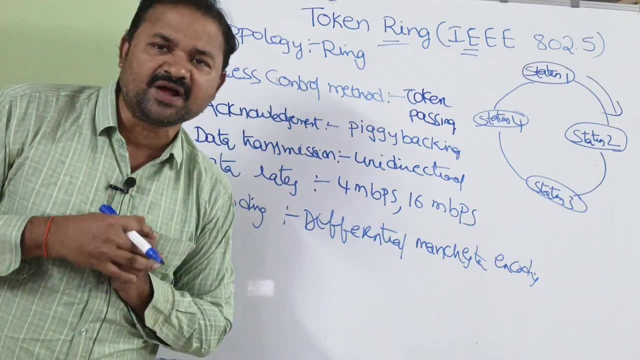 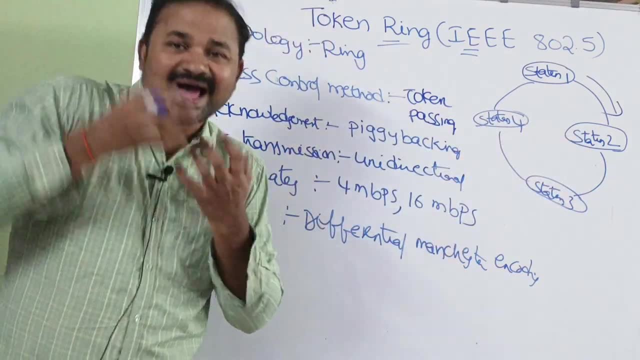 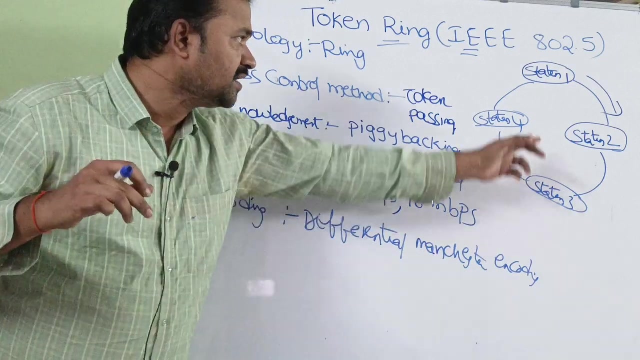 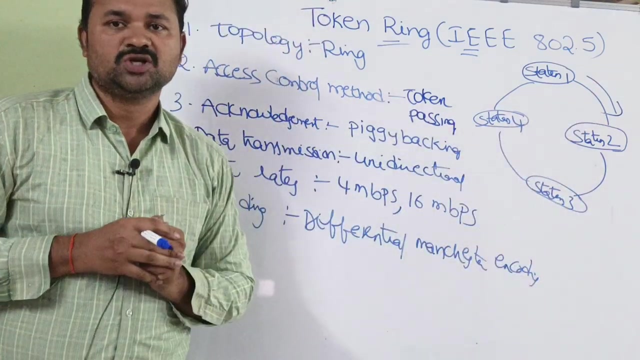 piggybacking acknowledgement. so piggybacking acknowledgement means, uh it let us assume that a station 2, so station 2- received some data from the station 1, so now, in addition to providing the acknowledgement for the station 1, station 2 can also transmit the data. so that is called as the. 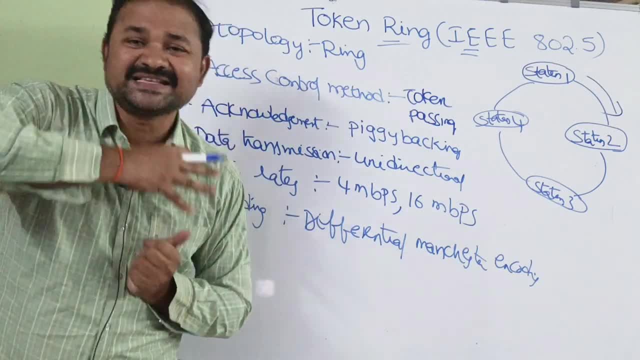 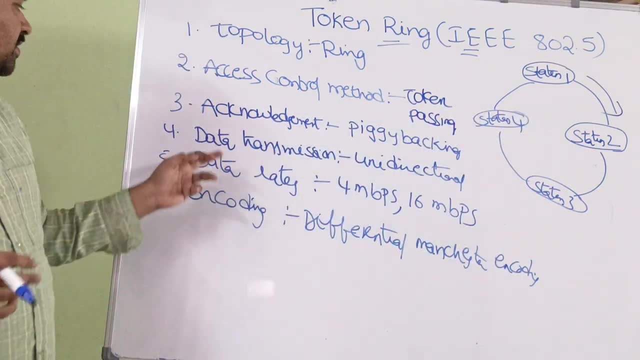 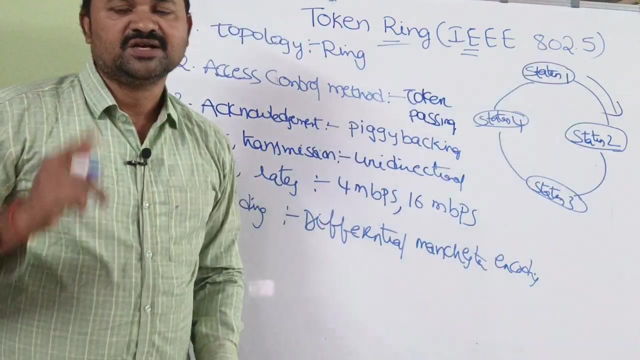 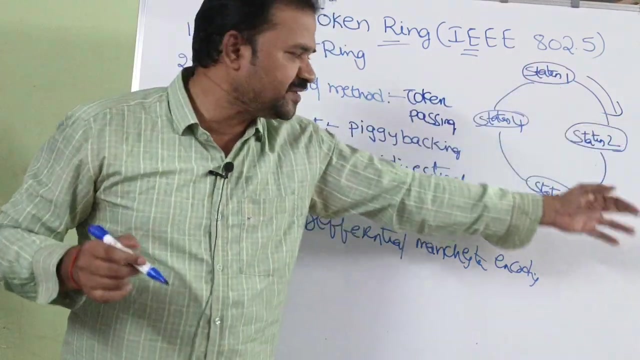 piggybacking. so piggybacking means transmission of the data along with acknowledgement, along with acknowledgement. and the next one is data transmission. here the data will be transmitted in unidirectional, so in only one way the data will be transmitted. so from station 1 to station 2, the data will be transmitted. next,